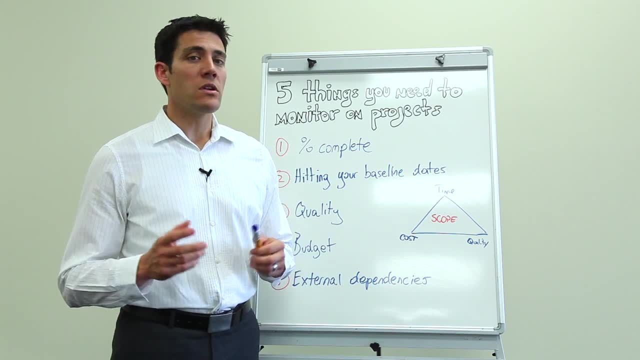 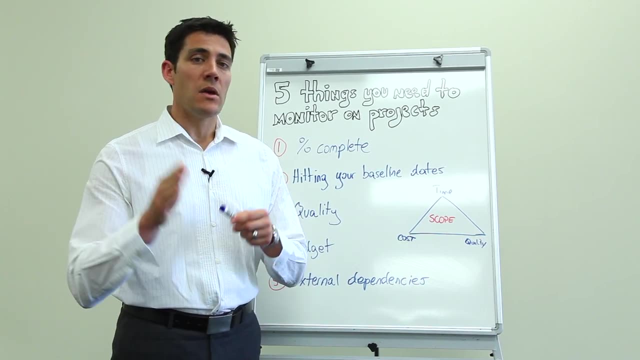 test plan are also due, and when they are delivered, It's not good enough just to say that I'm 100% complete. Yet I'm two weeks late. You're going to end up having a knock-on effect for not being able to deliver on time to other components of perhaps a larger program of work. So it's. 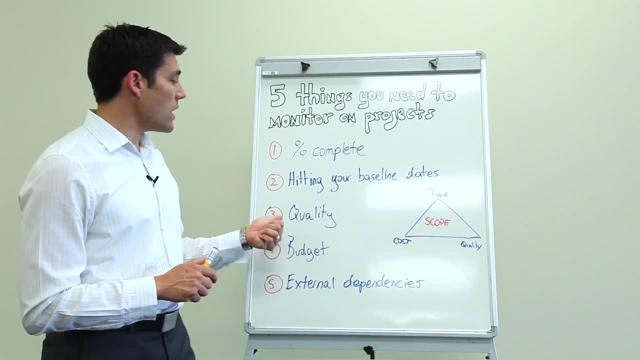 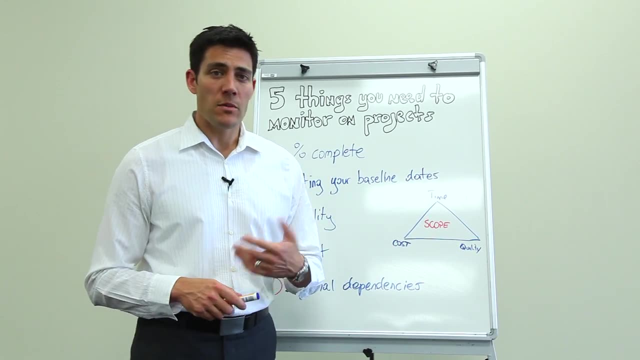 really important to keep an eye on hitting your baseline dates. Next, quality: It's no good to deliver something into production that is of poor quality and fails the day after. What would it be like if someone built a building with a shonky? 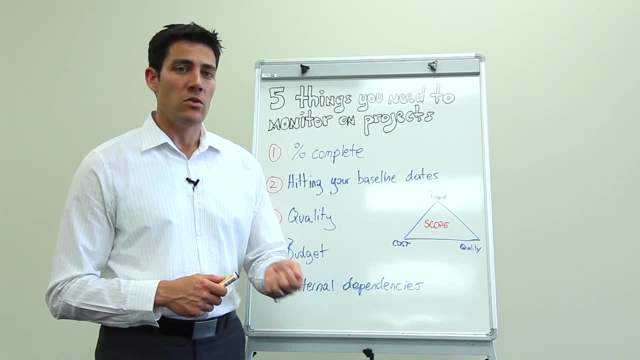 front door and they go over to hand over the keys to the new tenant or the new owner of the building and they can't get through the front door. It's no good. They hit it on time. It was 100% complete. 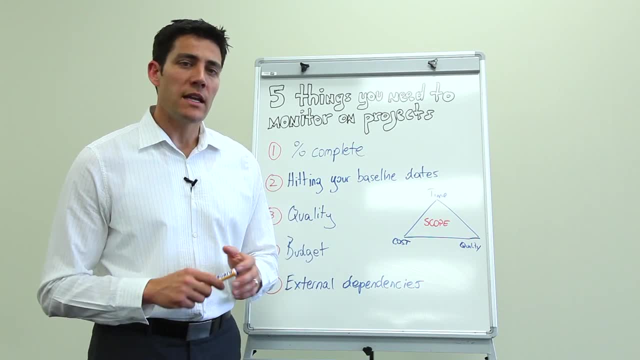 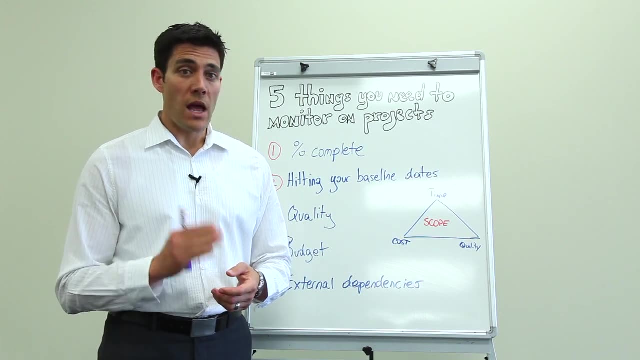 But the quality of that outcome was less than desirable, So you've got to keep an eye on your quality. There's many different ways to do that. You can do it through peer reviews whilst the project is underway. You can do it through health checks, which might occur. 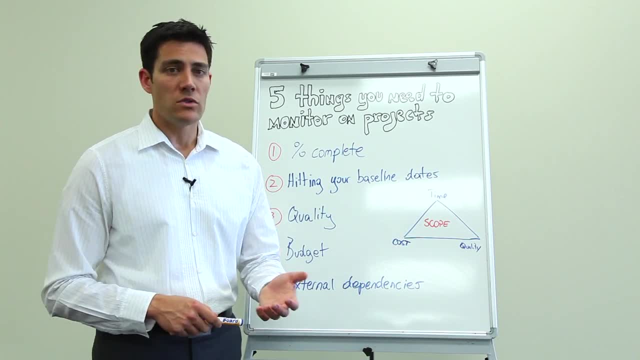 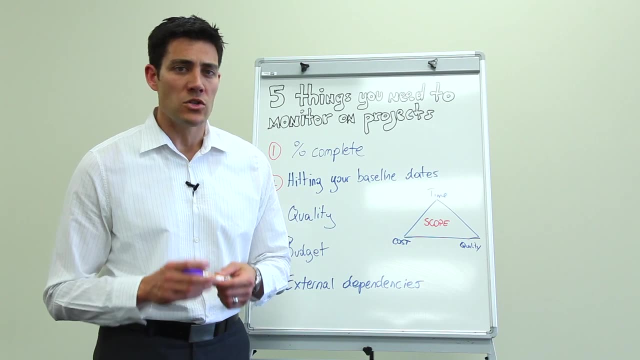 a third of the way through the project and another third of the way through that. Do it through design reviews, testing scripts and test results. There's a good number of ways for you to make sure that you manage your quality on your project. Make sure as 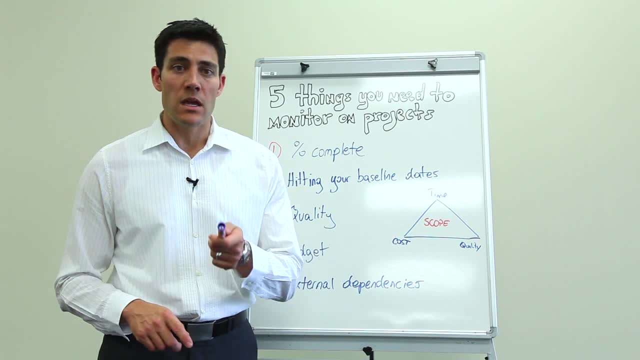 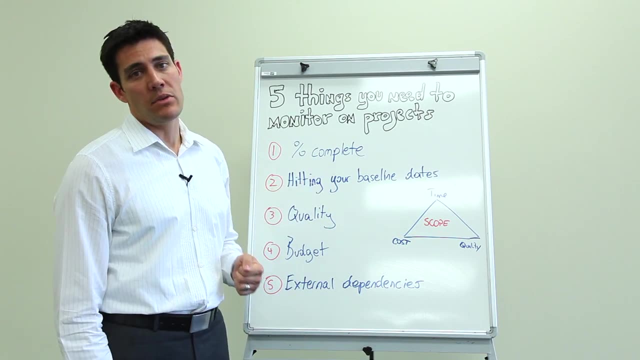 a PM. don't delegate that to your technical lead. Make sure you are keeping a vested interest in how the quality of your project is. Lastly, budget: If you are managing percent complete, you are hitting your baseline dates and the quality is fit for purpose for what you've been pulled in to do. then, of course, 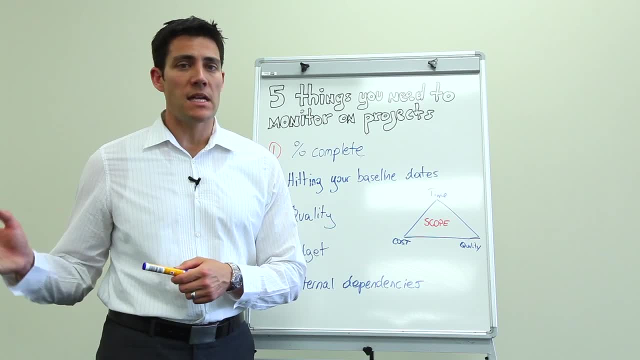 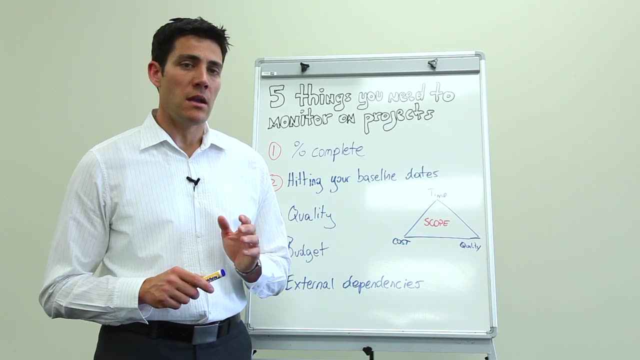 your budget should be on track. It's not always the case. Sometimes some tasks and projects run a little bit hot. Sometimes they run a bit low and a little bit lean. It's important as a project manager to make sure that you manage and maintain a good eye on the cost. 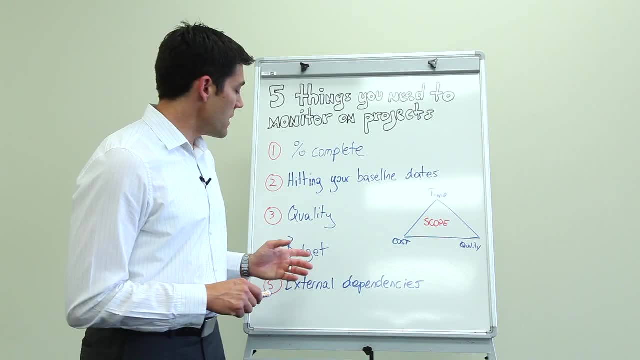 of your project and what your burn rate is against what you expected. It's always embarrassing when you go in front of the steering committee to go and ask for more money. You have to ask for more money when they don't know about it and you haven't warned them. 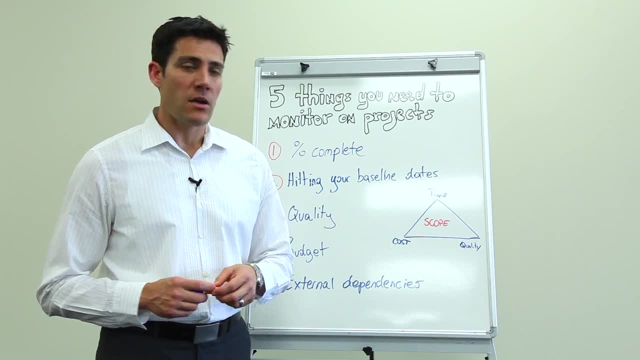 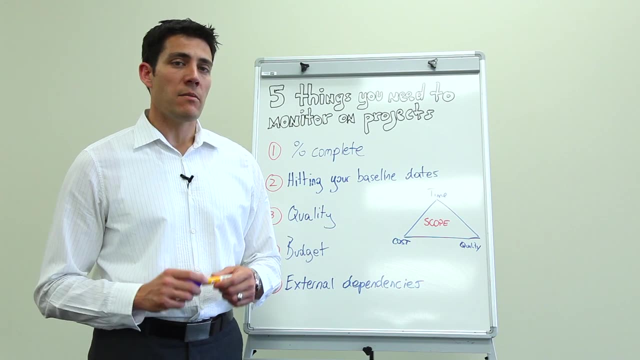 about that particular change request that you have to do. Make sure you keep an eye on your budget. Lastly, external dependencies. These are always something that come out of left field and you need to manage them very, very closely. The ones that will normally get you are the. 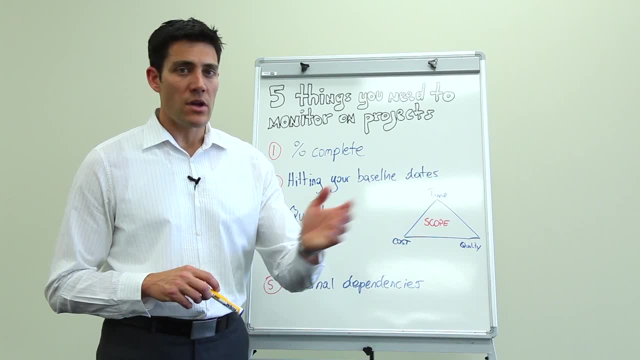 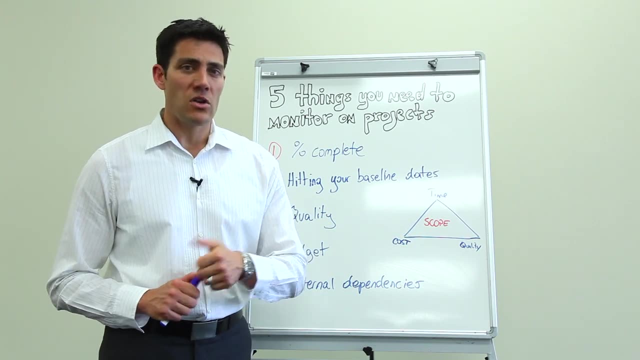 ones that are being delivered internally through an organization. Let's say, another project team or another functional group has got to deliver to you a set of requirements. Well, if you give them a get out of jail card for not delivering to the dates that you asked,